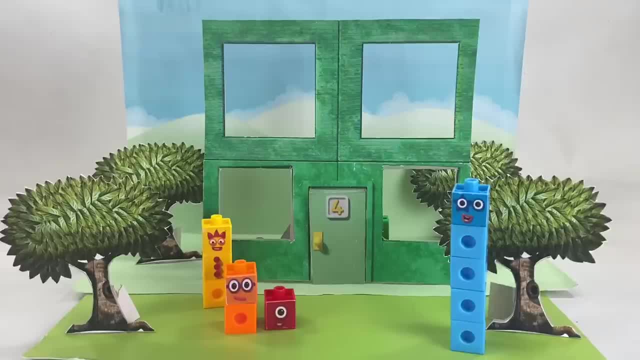 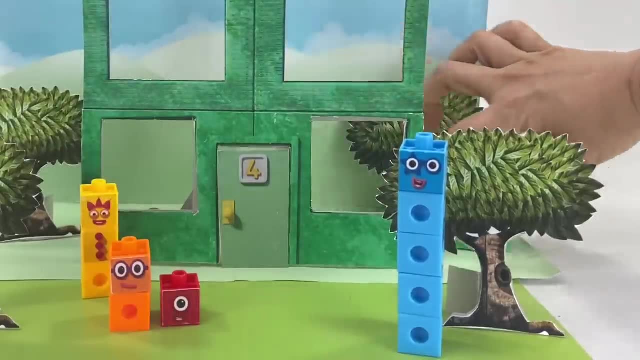 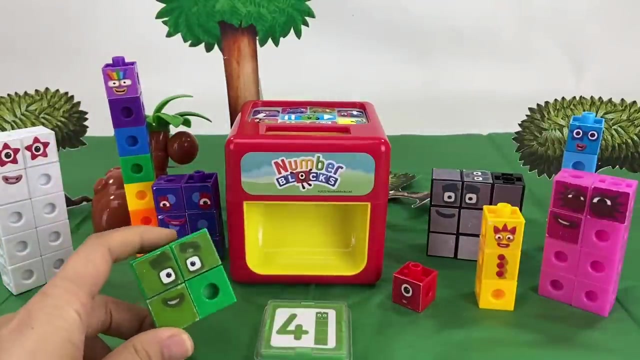 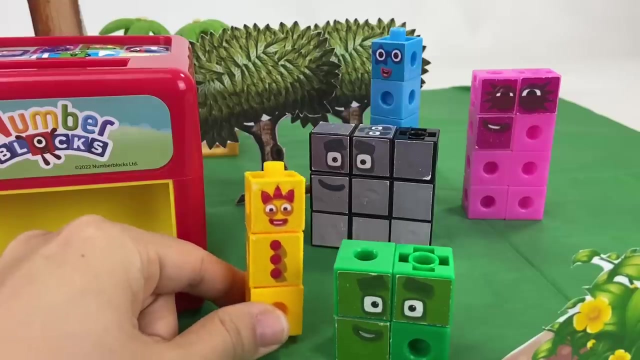 Ooh, That's me. Try to find me, Found me. I'm over here. Brilliant, I am four. I am one. two, three, four, Four blocks Me, Me, It's my turn. Can you find number block five. 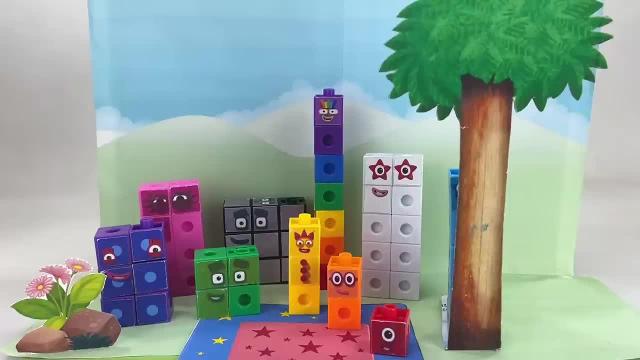 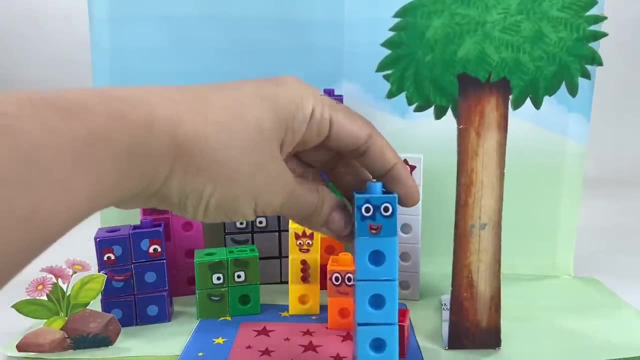 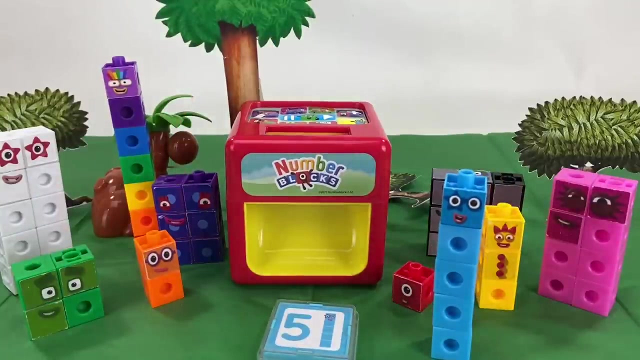 Ooh, It's high time for high five. Find me Here. I am Good job. I better change that hiding place. It's becoming too easy. Brilliant, I am five. I am one, two, three, four, five, Five blocks. Can you find number block eight? 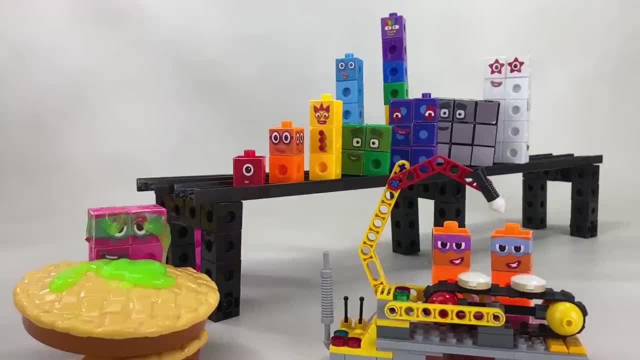 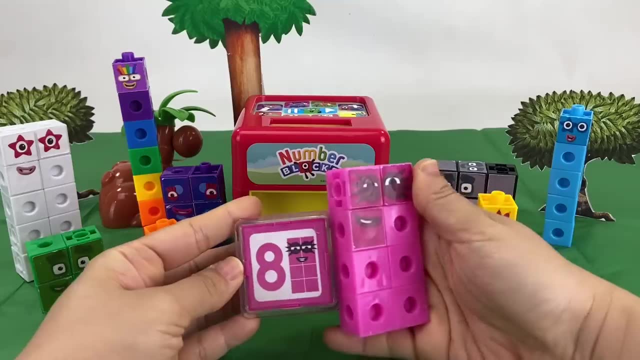 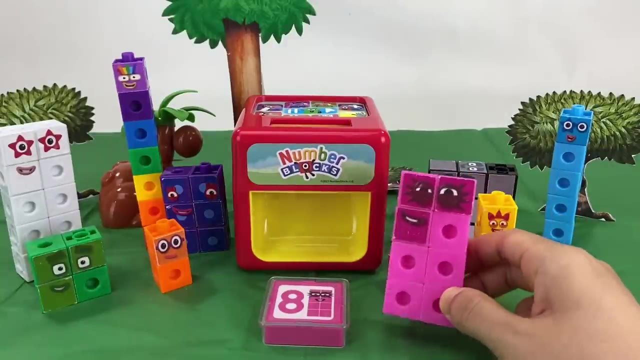 That's me Octoblock hide One, two, three, four, five, six, seven, eight. Hide. Can you see me Here? I am Brilliant. I am eight, One, two, three, four, five, six, seven, eight, Eight blocks. 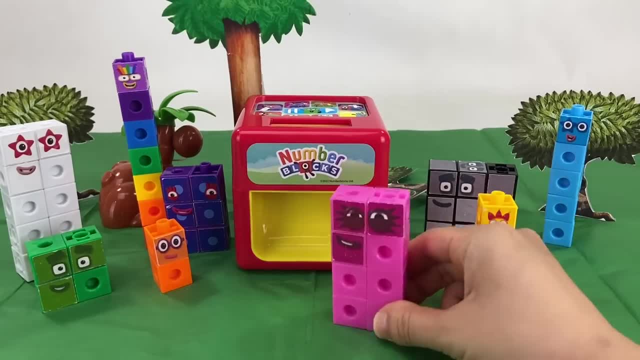 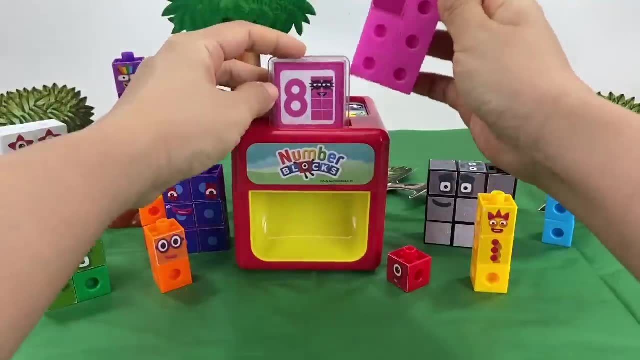 Can you find number block eight? Ooh, It's me again. Find me Here, Brilliant, I am eight. One, two, three, four, five, six, seven, eight. Hide One, two, three, four, five, six, seven, eight, Eight blocks. 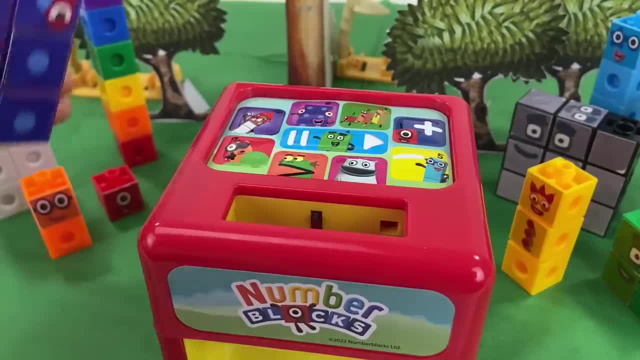 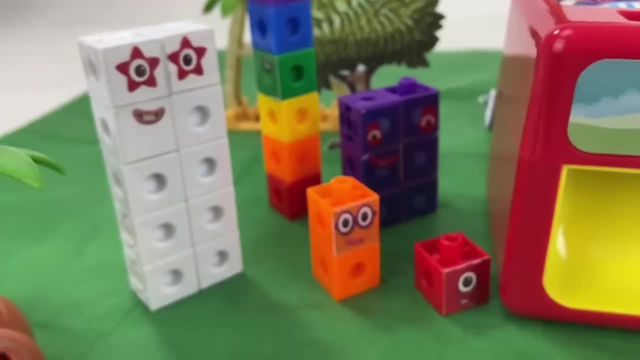 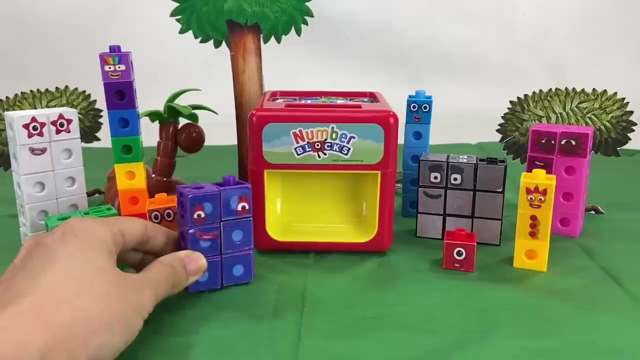 Want to play a different game. Press another game on top of the cube: Number magic. Want to find out how many blocks we would have if we added two number blocks together. Put them in the cube to find out. Ooh, That sounds fun. Who wants to try? 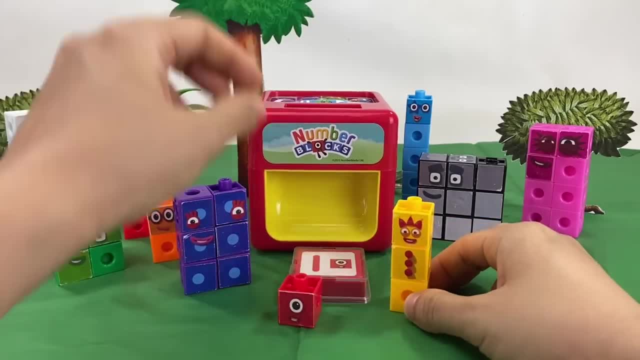 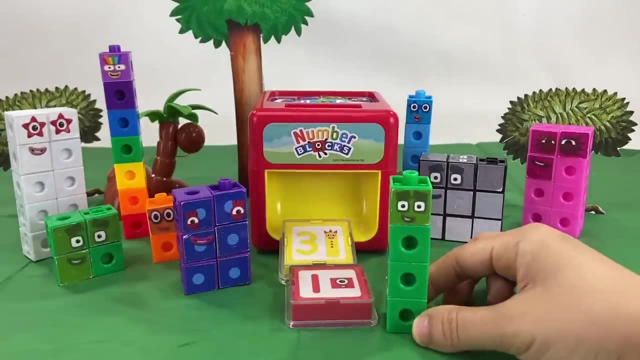 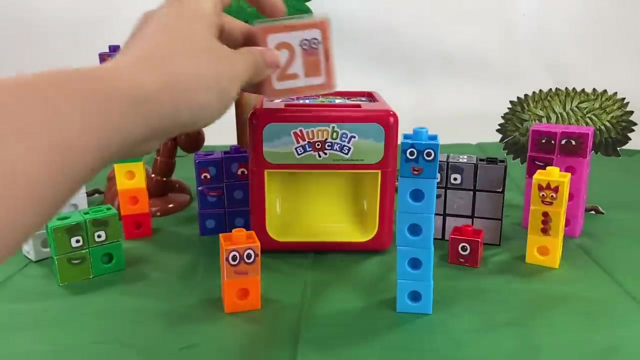 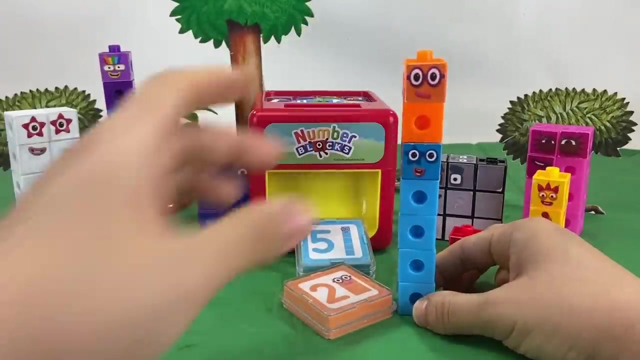 I'll try Me Me. One plus eight Equals four, Seven. Well done, I'll give it a go, And me too. Two plus five Equals seven. Want to play a different game. Press another game on top of the cube. 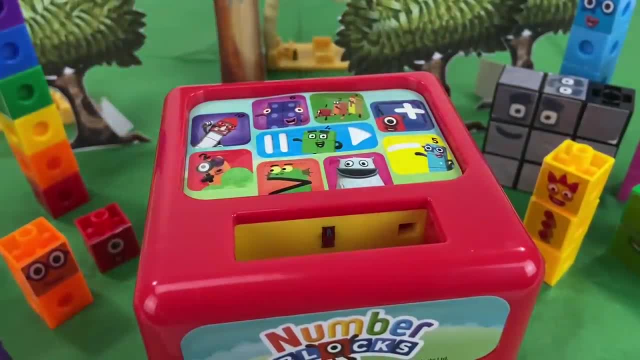 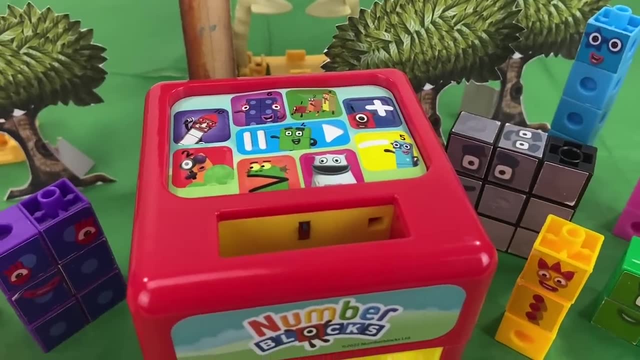 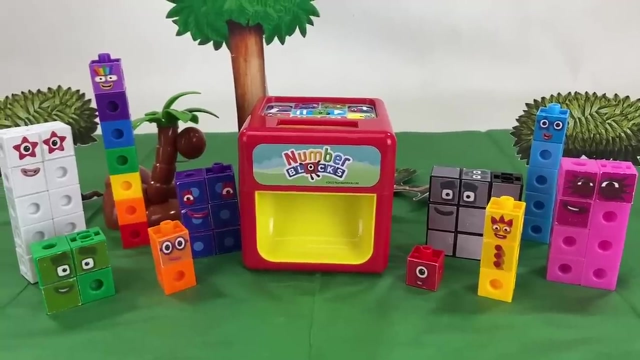 A number block has gone to play with Big Tom. Do you know which number block is missing? Let's find out. One, two, three, four, five, six, seven, eight, nine, ten. Which number block is missing? 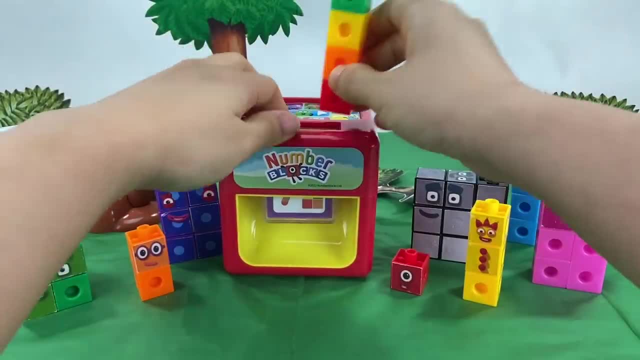 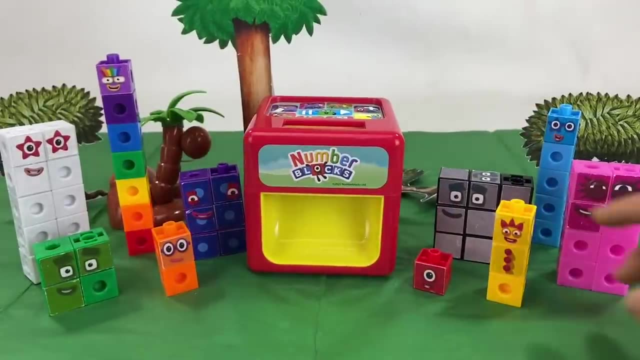 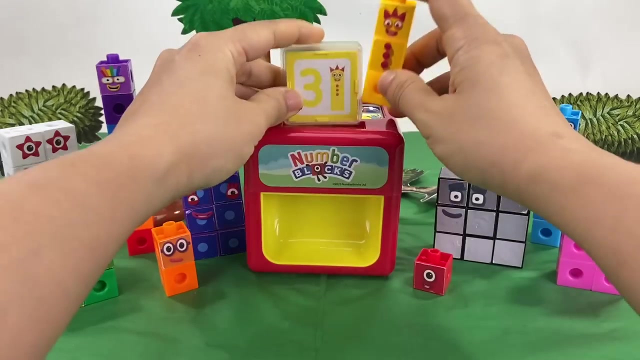 Seven, That's me, I am seven, That's lucky. One, two, three, four, five. Which number block is missing? Missing Why? that's me, of course. Put another block into the cube. I'm seven. 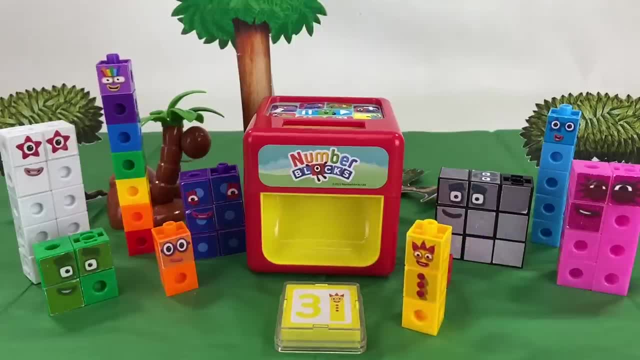 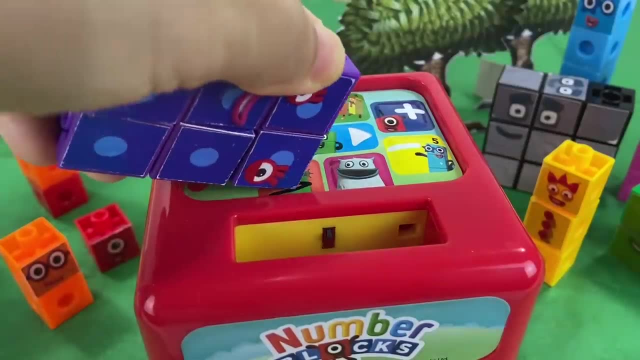 Number three is missing. Look, I did it, Well done. Want to play a different game? Of course, Press another game on top of the cube. Let's meet Bloxzilla. See Bloxzilla, They like big things. 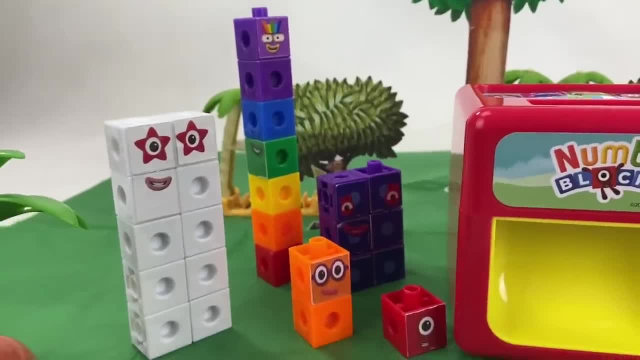 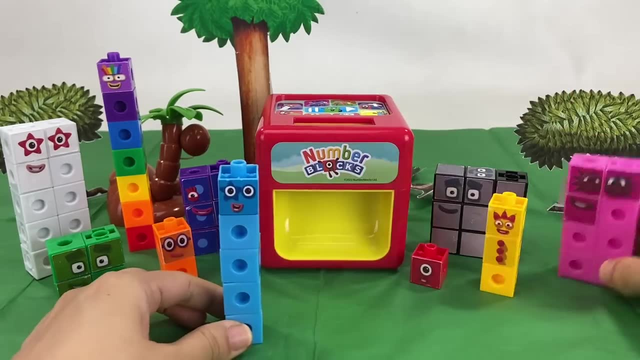 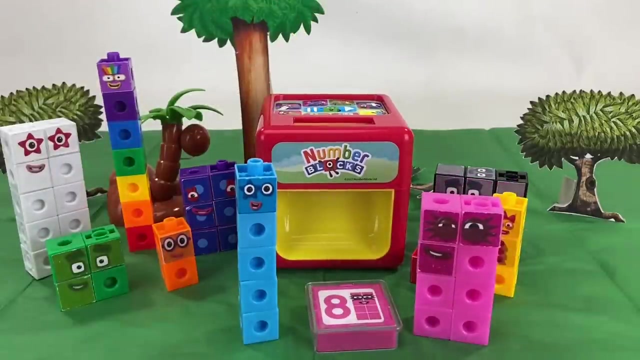 Which number block is bigger. Greater means bigger, Bigger. so me like pick up number block 5 and number block 8.. It's me, of course I'm bigger. Well done, Yes, number block 8 is bigger. Me like big things. 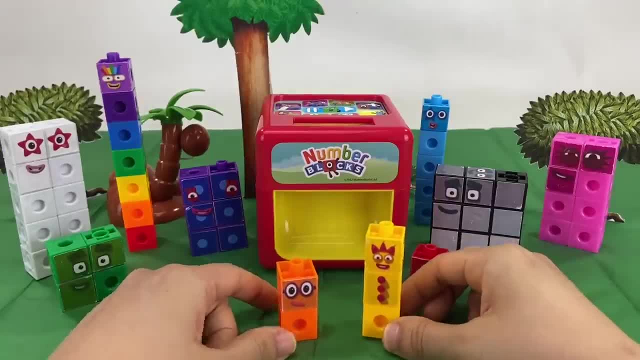 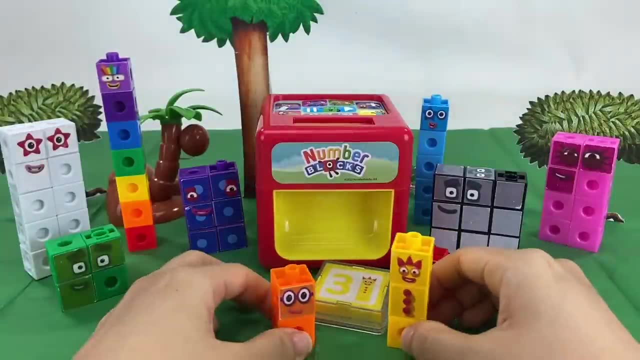 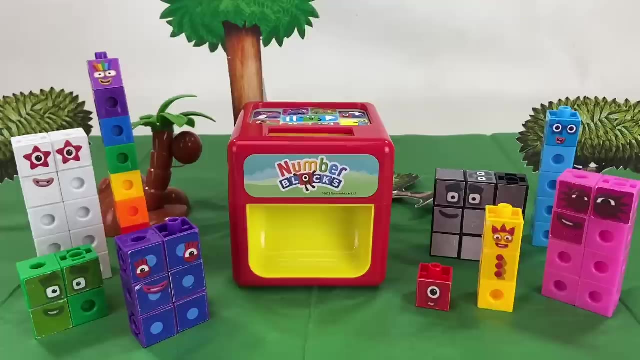 Pick up number block 2 and number block 3. Place the bigger number block in the queue. Of course it's me. I'm the biggest. Well done, Yes, number block 3 is bigger. Me, like big things, Want to play a different game. 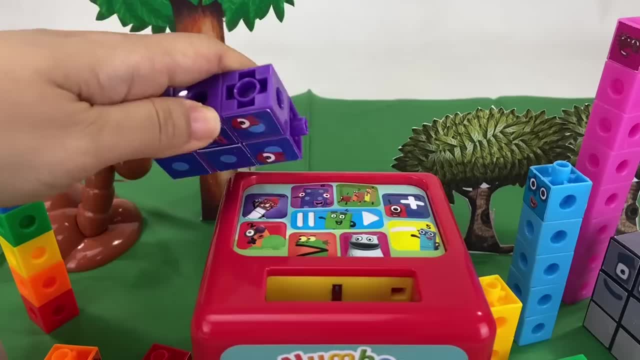 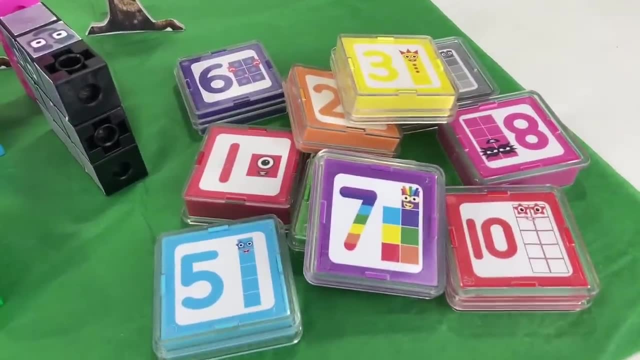 Press another game on top of the cube. I love all these games. Let's find out some fun number facts. Place the number block in the queue to get started. I'll give it a go. I am 2.. How do you do? 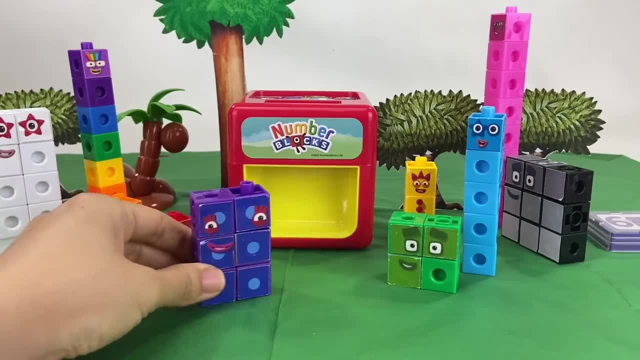 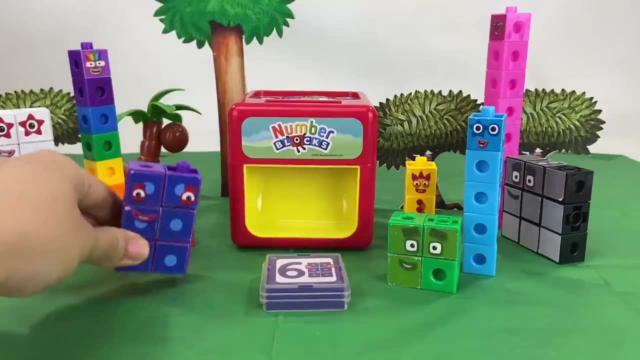 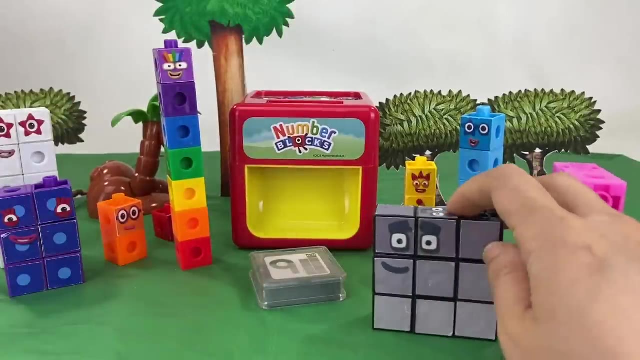 I love things that are too old. I'm next. Number 6 is in the mix. I am 6 in the mix. Time for rhymes and skips and tricks. I'll go next before I have a tickly nose. I'm 9 and I feel fine.